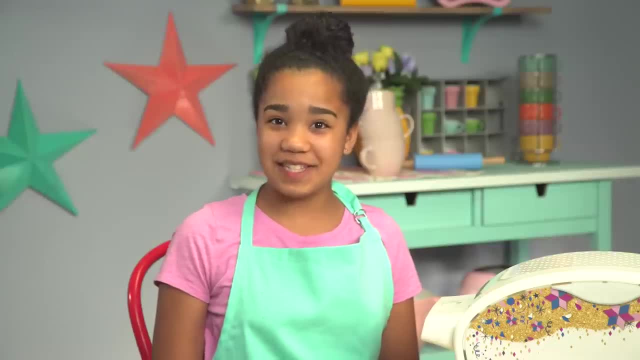 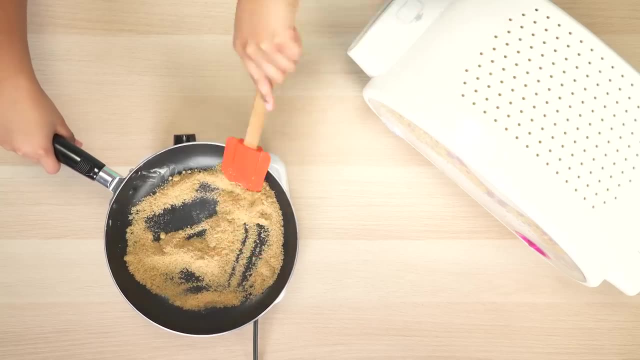 and a half cup of breadcrumbs. First, turn on your Easy Bake Oven. Mix the breadcrumbs with butter in a pan. Mix the butter with butter in a pan. Add the salt and pepper to the flour and dump it in. Add the salt and pepper to the flour and dump it in. 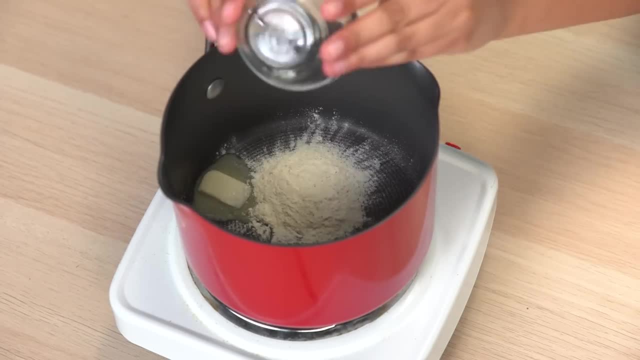 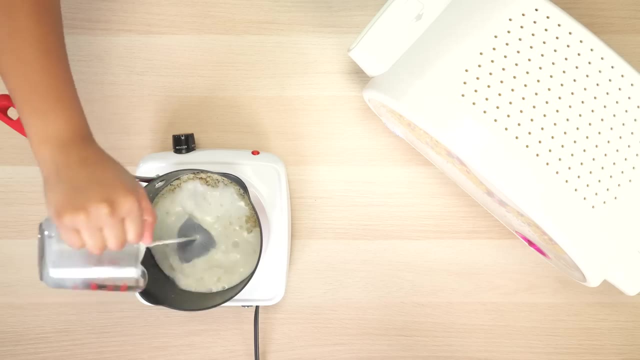 Add the salt and pepper to the flour and dump it in. Mix the salt and pepper with the flour and dump it in. Stir it up with a whisk. Keep stirring till it's blended. Pour the milk and sour cream in. Stir until it's boiling. 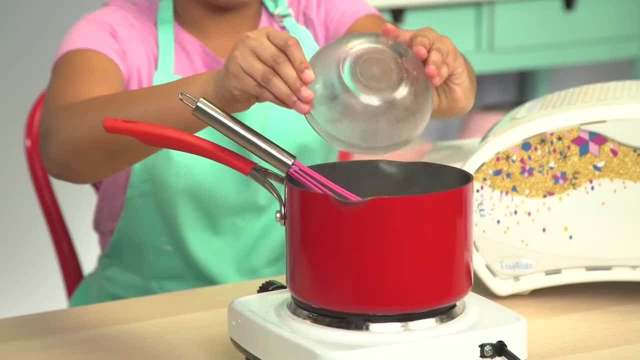 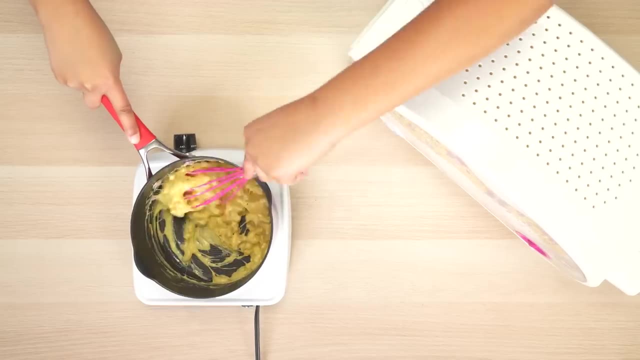 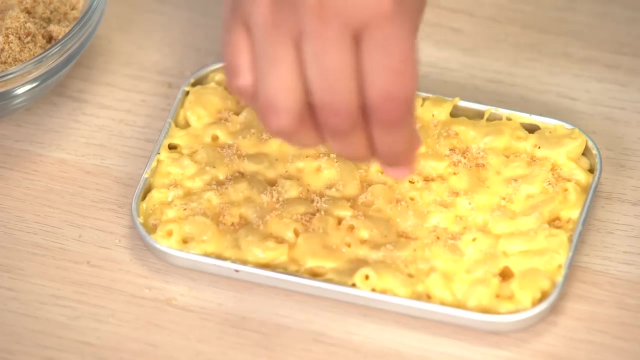 Now for the cheesy part. add your cheese, Turn off the heat. Add the noodles and stir it up. Put the mac and cheese into an Easy Bake Oven pan. Sprinkle it with breadcrumbs. Time for this mac and cheese to bake. 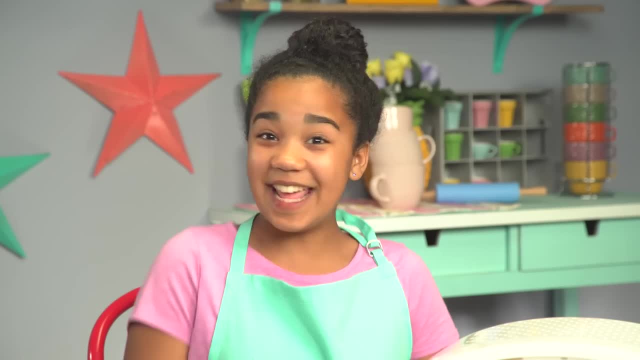 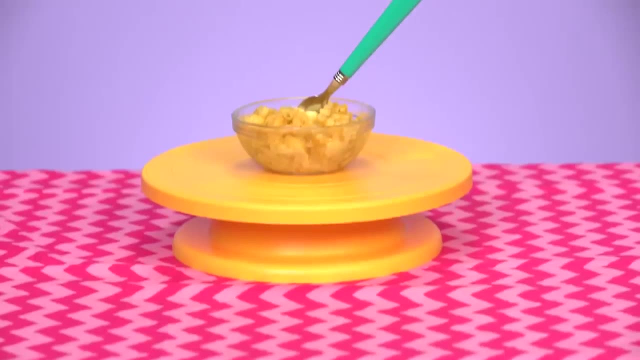 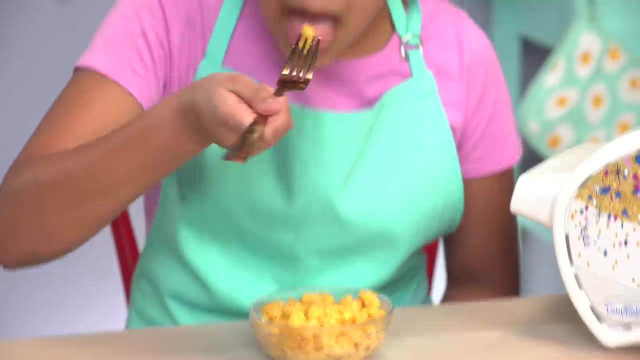 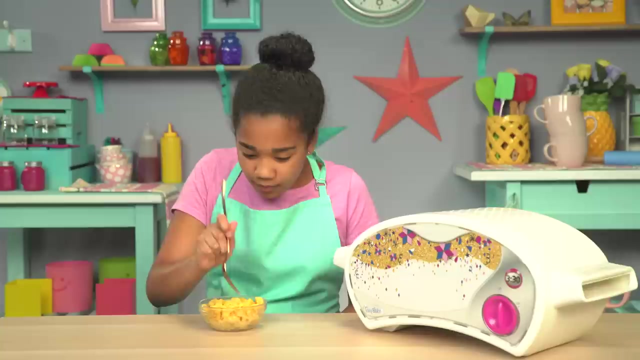 Bake for 20 minutes till the top is golden. It's ready. So how does mac and cheese from an Easy Bake Oven taste? Bake for 20 minutes till it's golden. Oh my gosh, so good And cheesy. For our second challenge, we'll be doing something with 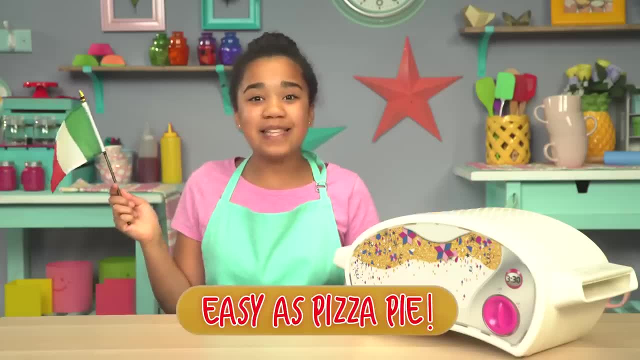 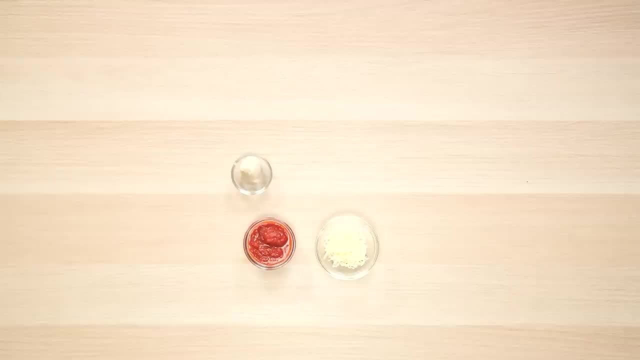 an Italian flair. Here's how to make my Easy As Pizza pie. To make this, you'll need pre-made pizza dough, pizza sauce, mozzarella cheese, Parmesan cheese and one slice of pepperoni. Turn on the Easy Bake oven. 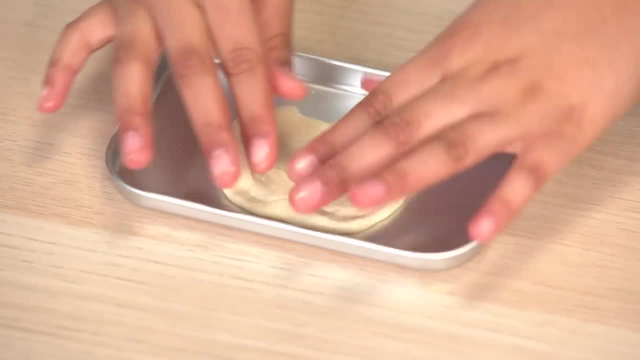 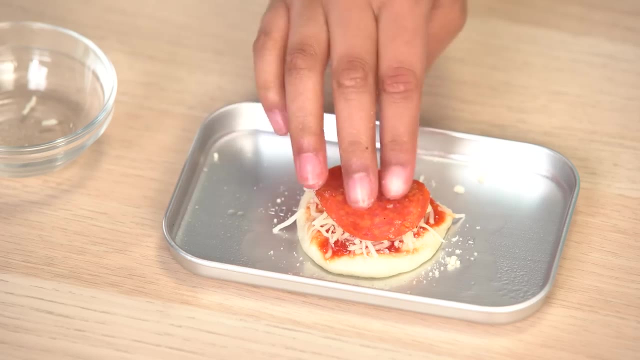 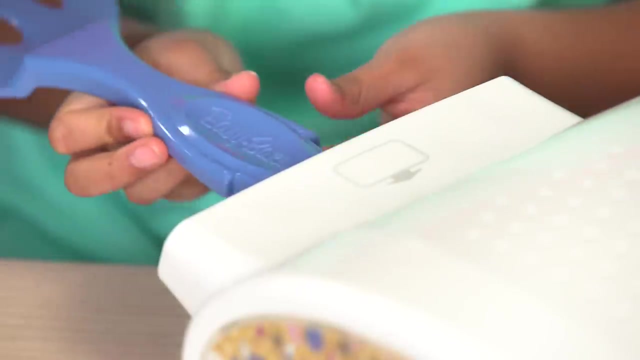 Use your fingers to press out the pizza dough on the Easy-Bake oven tray. Add pizza sauce, cheeses and your pepperoni. Bake it in the oven for 20 minutes. It's got to be flat to go in Pizza time. 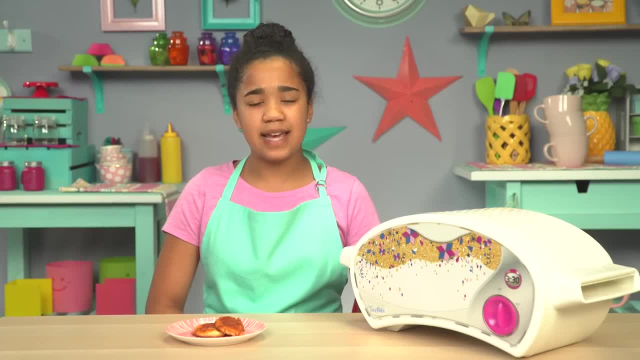 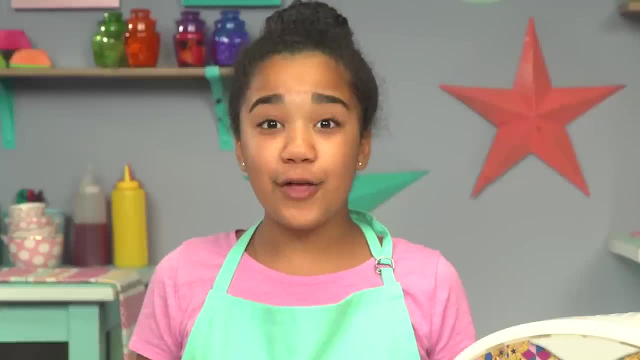 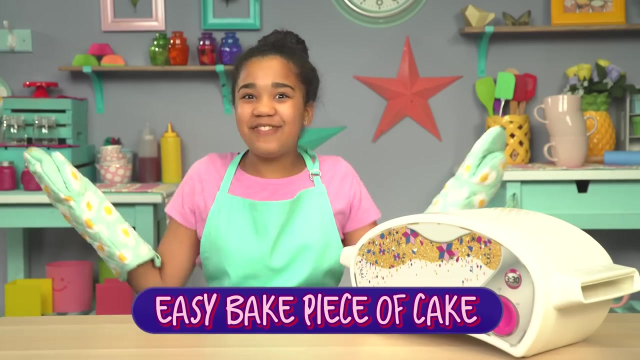 Now, how does Easy-Bake oven pizza taste Delicious, y'all so mwah. For our third challenge, we're going to need a sweet treat. Here's how to make my Easy-Bake piece of cake. To make this, you'll need a pre-made box of cake mix.